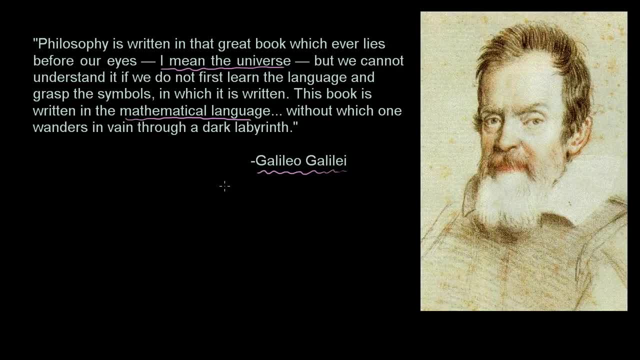 you know, the philosophy of the universe is written in mathematics. But let's start with a very concrete, simple idea. But we'll keep abstracting and we'll see how the same idea connects across many domains in our universe. So let's just say we're at a store. 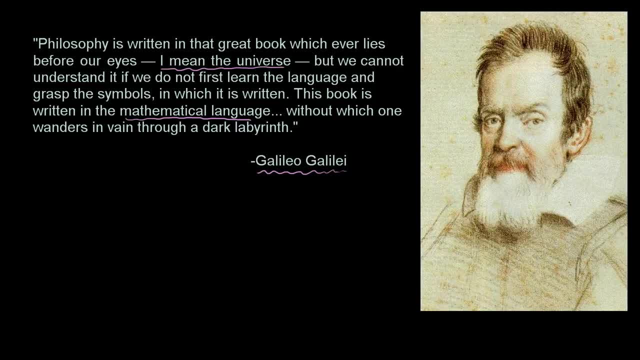 And we're going to buy something And there's a sale. The sale says that it is 30% off And I'm interested. I don't shop at too fancy stores, So let's say I'm interested in a pair of pants. 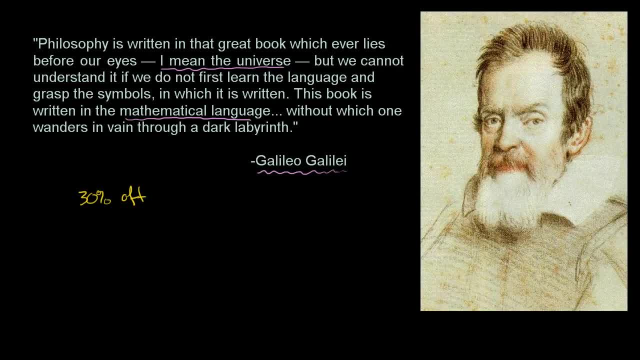 And the pair of pants- before the sale even, is about $20.. And that is about how much I spend on my pants. So I'm interested in a $20 pair of pants. But it's even better: There's a 30% off sale on these pants. 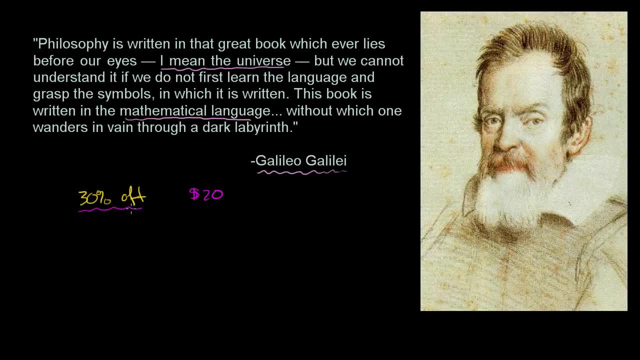 Well, how would I think about how much I'm going to get off of that $20?? And this isn't algebra yet. This is something that you've probably had exposure to. You would multiply the 30% times the $20.. So you would say your discount is equal to. 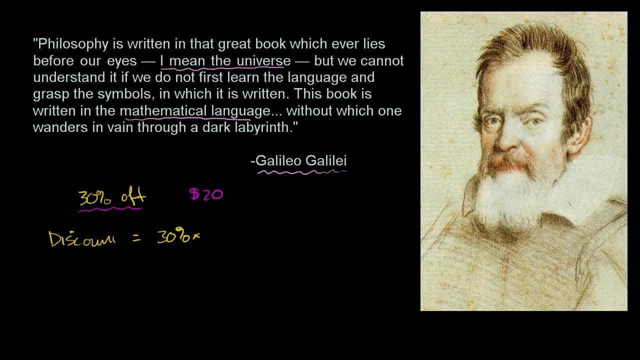 you could write it as 30% times $20.. I'll do the $20 in purple, Or you could write it. if you wanted to write this as a decimal, you could write this as 0.30 times $20. And if you were to do the math, you would get $6.. 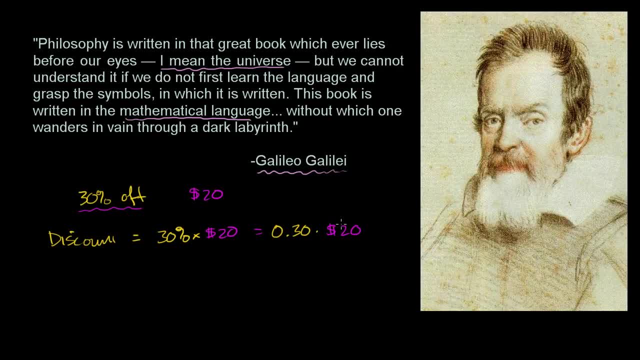 So nothing new over there. But what if I want to generalize it a little bit? That's the discount on this particular pair of pants. But what if I wanted to know the discount on anything in the store? Well then I could say: well, let x be the price. 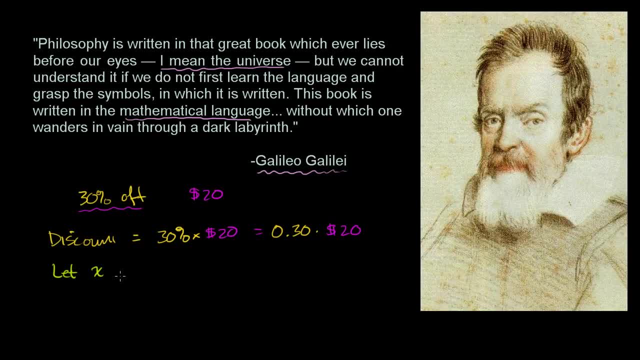 Let me do this in a different color. So I'm just going to make a symbol. Let x be the price of the product I want to buy, The non-discount price, The price of the product in the store. So now, all of a sudden, we can say that our discount. 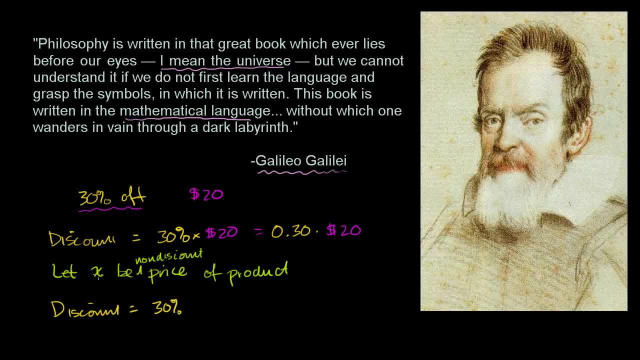 is equal to 30% times x. Or if we wanted to write it as a decimal, we could write: if we wanted to write 30% as a decimal, we could write 0.30 times x. Now, this is interesting. 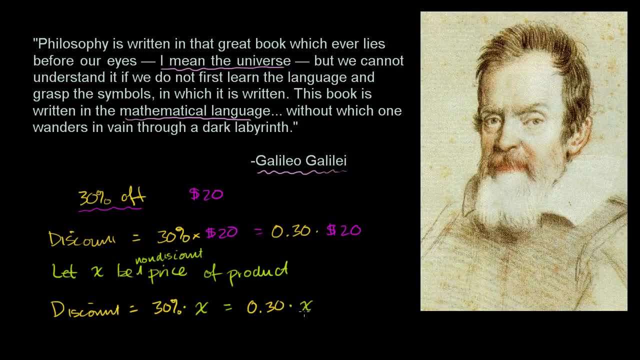 Now you give me the price of any product in the store and I can substitute it in for x, And then I can essentially multiply 0.3 times that and I would get the discount. So now, very slowly, we're starting. 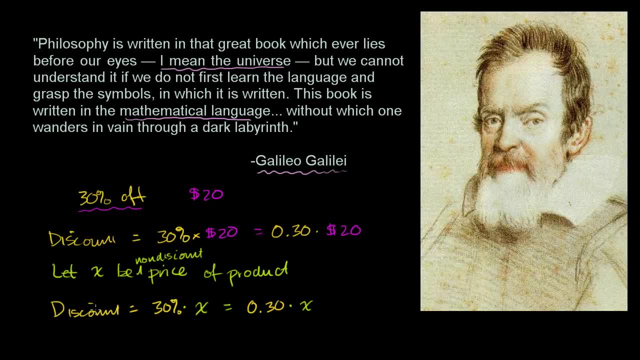 to get into the abstraction of algebra And we'll see that these will get much more nuanced and deep and, frankly, more beautiful as we start studying more and more algebraic ideas. But we aren't done here. We can abstract this even more. 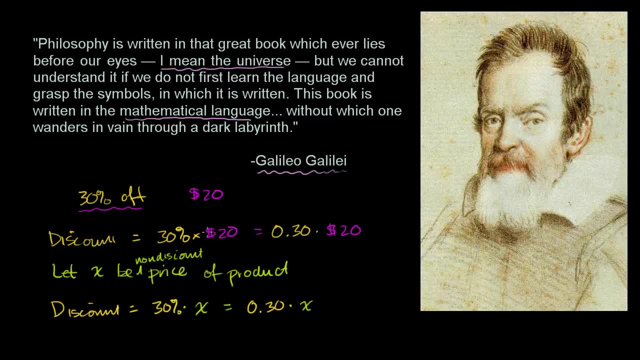 Over here we've said, We've generalized this for any product. We're not just saying: for this $20 product. If there's a $10 product, we can put that $10 product in here for x, And then we would say 0.30 times 10.. 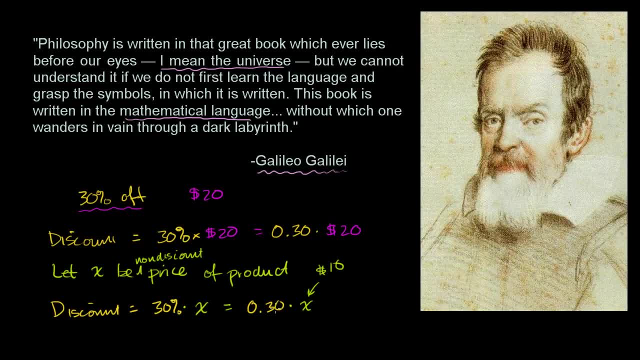 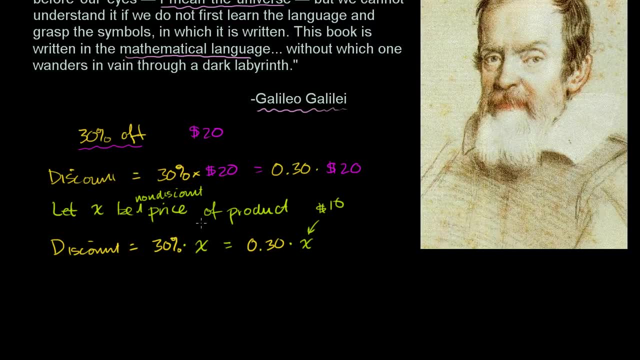 And the discount would be $3.. It might be a $100 project. Then the discount would be $30.. But let's generalize even more. Let's say: well, what is the discount for any given sale when the sale is a certain percentage? 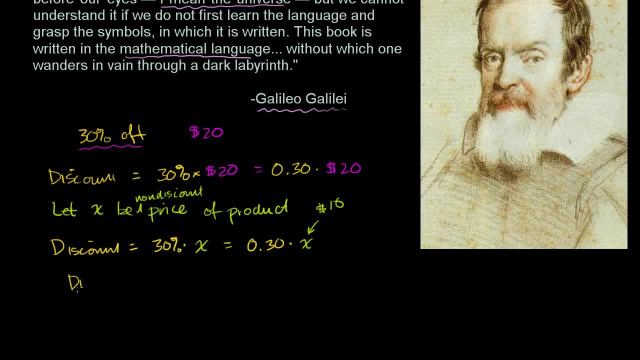 So now we can say that the discount- Let me define a variable. Let's let m equal, or I'll say p, just so it makes sense- p is equal to the percentage off. Now, what can we do? Well, now we can say that the discount is. 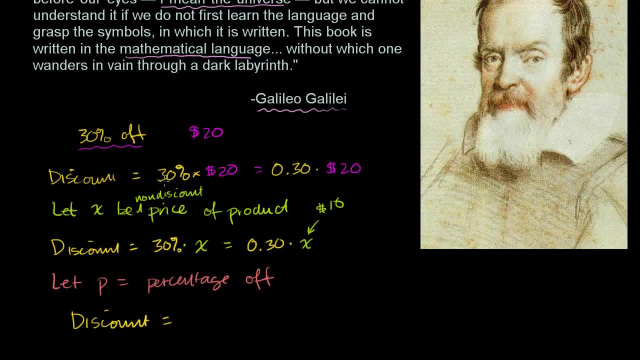 equal to the percentage off. In these other examples we were picking 30%, But we can say now: it's p, It's the percentage off, It's p. That's the percentage off times the product in question, times the price, the non-discount price. 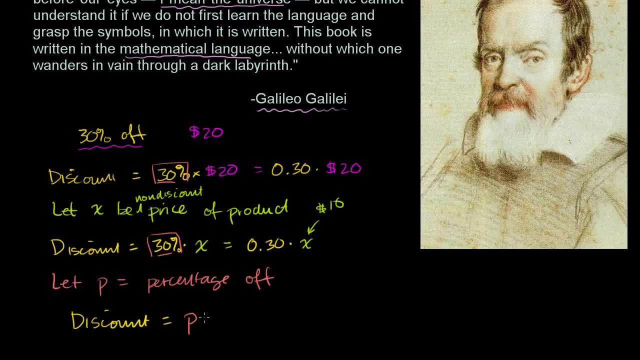 of the product in question. Well, that was x. The discount is equal to p times x. Now this is really interesting. Now we have a general way of calculating a discount for any given percentage off and any given product- x- And we didn't have to use these words and these letters. 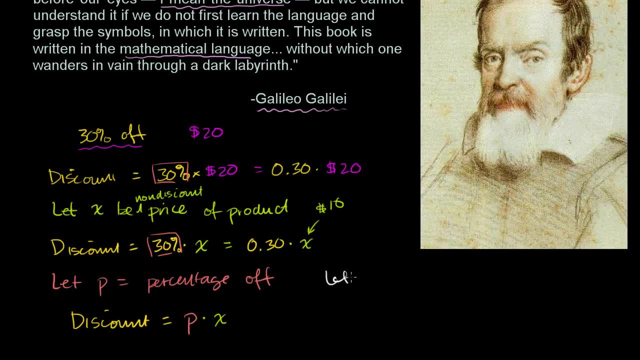 We could have said: let y equal the discount, Let y equal the discount, Let y is equal to the discount. Then we could have written the same underlying idea. Instead of writing discount, we could have written: y is equal to the percentage off p times the non-discount price. 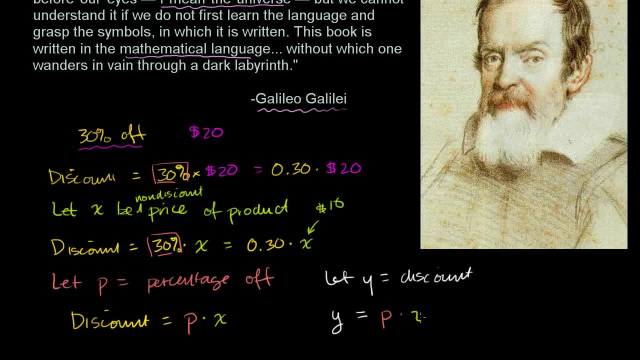 of the product times x, And you could have defined these letters any way you wanted. Instead of writing y there, you could have written a Greek letter, or you could have written any symbol there, as long as you can keep track of that that symbol represents. 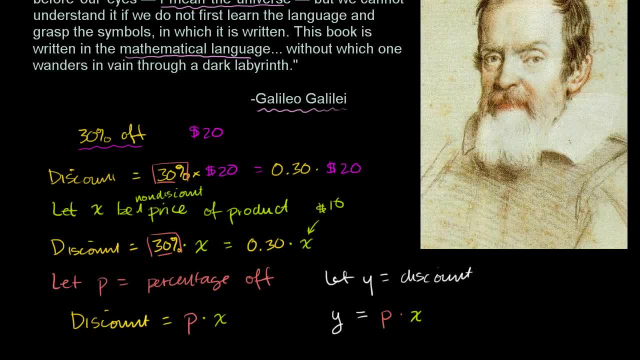 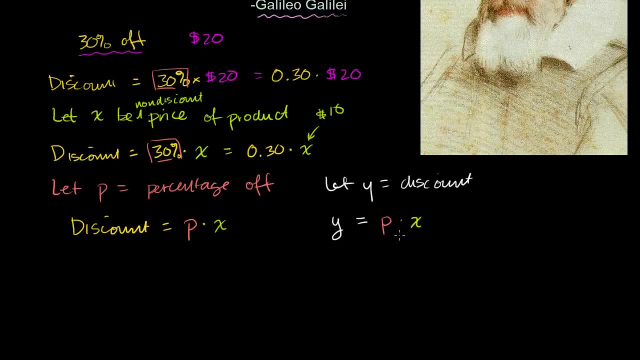 the actual dollar discount. But now things get really interesting, because we can use this type of a relationship, which is an equation. You're equating y to this right over here. That's why we call it an equation. This can be used for things that are completely unrelated. 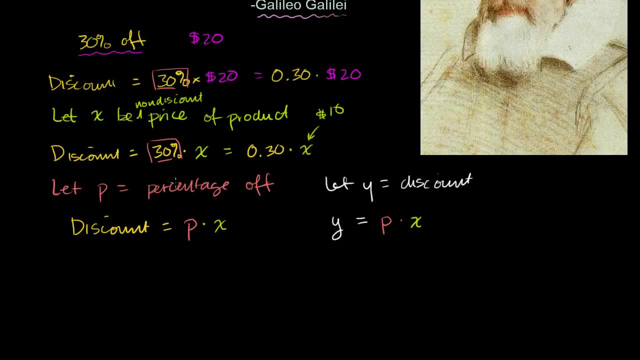 to the discount price at the store over here. So in physics you'll see that force is equal to mass times acceleration. The letters are different, but these are fundamentally the same idea We could have. let y is equal to x. This is equal to force. 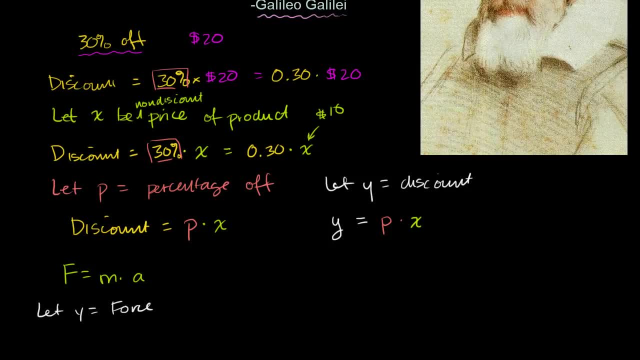 We could let: y is equal to force And m is equal to, or mass is equal to p. So let me write: p is equal to mass, And this wouldn't be an intuitive way to define it, But I want to show you that this is the same idea. 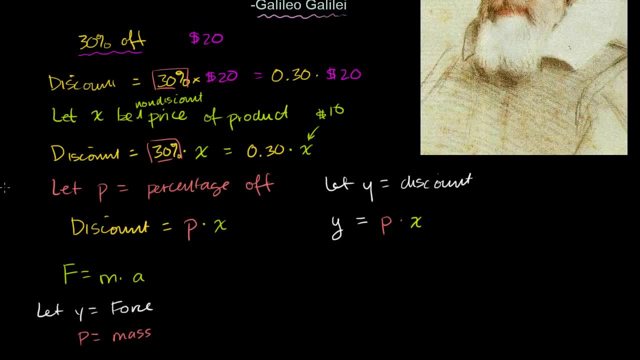 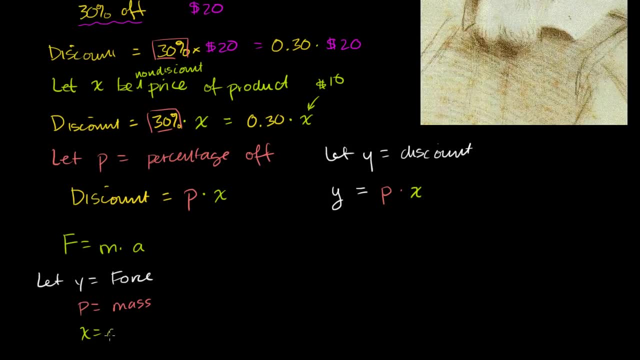 the same relationship, but it's being applied to two completely different things. And we could say: x is equal to acceleration. Well then, the famous force is equal to mass times. acceleration can be rewritten And it's really the same exact idea as y, which we've defined as force, can be equal to mass. 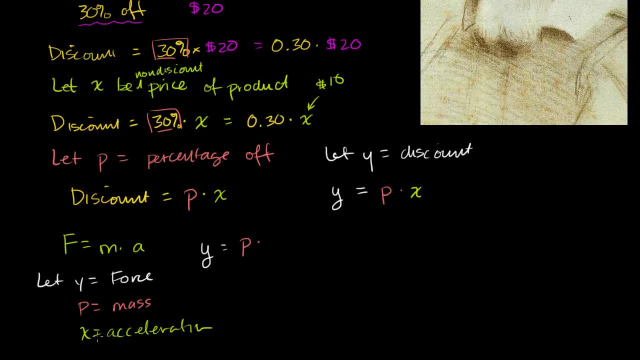 which we're going to use the symbol p, which is equal to p times acceleration, And we're just going to happen to use the letter x here, times x. Well, this is the exact same equation. We can see that we can take this equation. 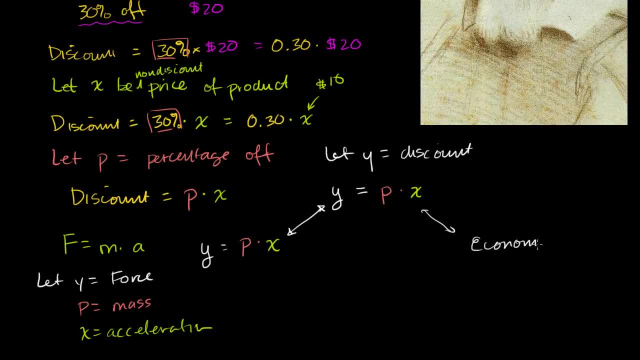 and it can apply to things in economics, Or it can apply to things in finance, Or it can apply to things in computer science or logic or electrical engineering or anything accounting. There's an infinite number of applications of this one equation. 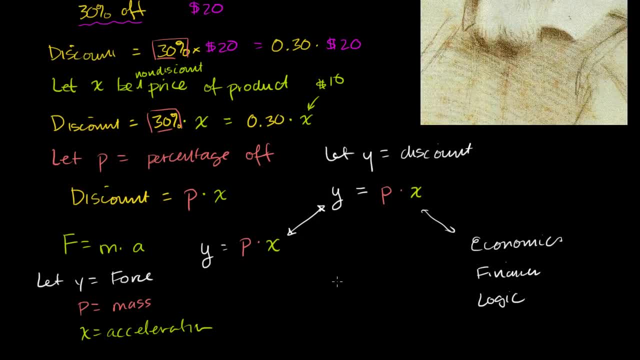 And what's neat about mathematics and what's neat about algebra in particular, is we can focus on this abstraction, We can focus on the abstract here And we can manipulate the abstract here. And what we discover from these ideas, from these manipulations can then 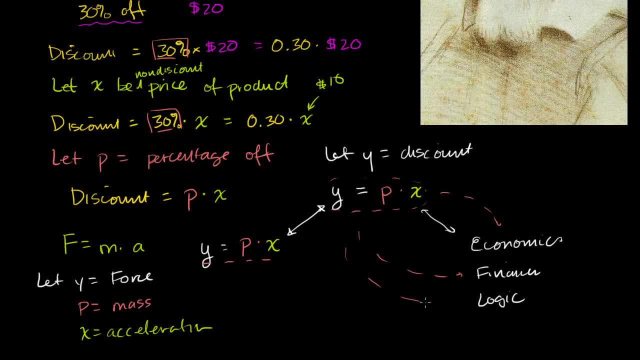 go into the abstract And we can manipulate the abstract here. It can be reapplied to all of these other applications, to all of them And, even neater, it's kind of telling us the true structure of the universe if you were to strip away all of these human definitions. 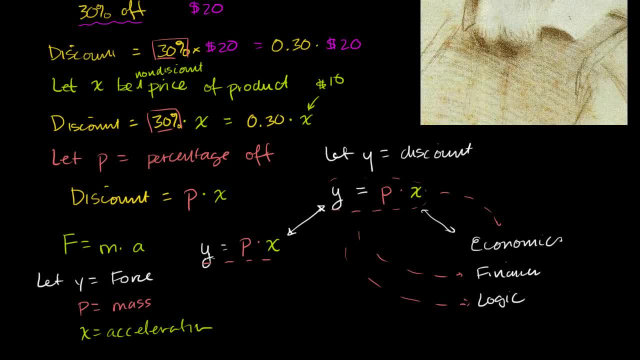 and all of these human applications. So, for example, we could say: look, if y is equal to p times x. so, literally, if someone said, hey, this is y and someone says, on the other hand, they say I have p times x, I could say, well, 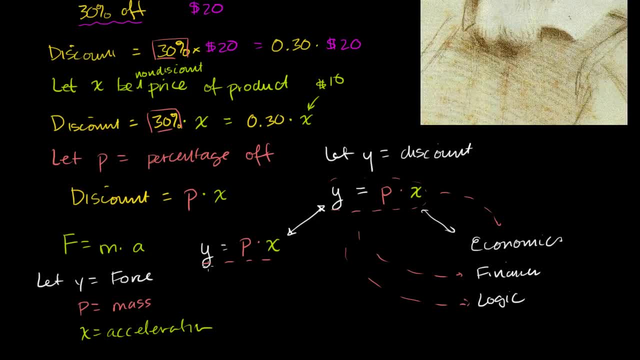 you have the same thing in both of your hands And if you were to divide one of them by a number, and if you wanted to divide one of them to still be equal, you would divide the other one by that number. So, for example, let's say we know that y is equal to p times x. 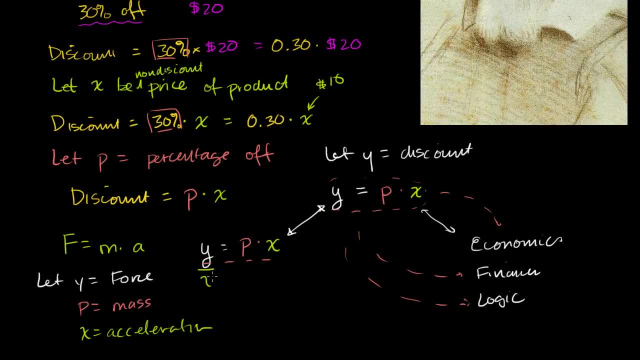 What if you wanted to have them both be equal and you say: well, what is y divided by x is going to be equal to? Well, y was equal to p times x. so y divided by x is going to be the same thing as p times x divided by x. 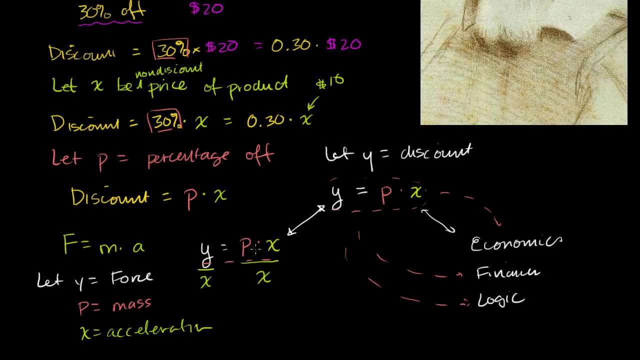 But now this is interesting because p times x divided by x. well, if you multiply by something and then divide by that something, your original number, if you multiply by 5 and divide by 5, you're just going to start with p or whatever this number is. 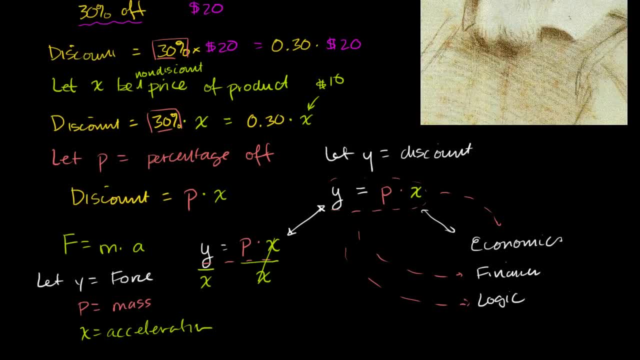 So those would cancel out. But we were able to manipulate the abstraction here and get: y over x is equal to p. Let me make that x green. y over x is equal to p. And now this has implications for every one of these ideas. 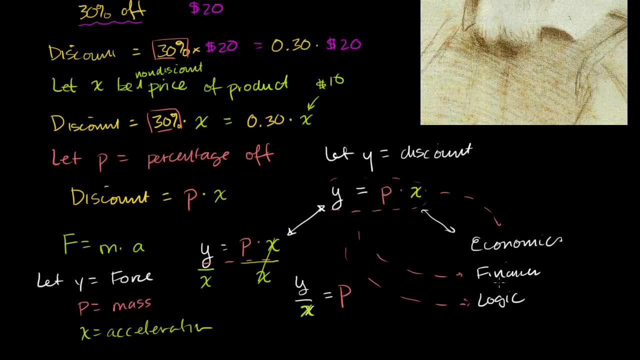 One is telling us a fundamental truth about the universe, almost devoid of any of these applications. But now we can go and take them back to any place that we applied, And the really interesting thing is we're going to find new. there are an infinite number of applications. 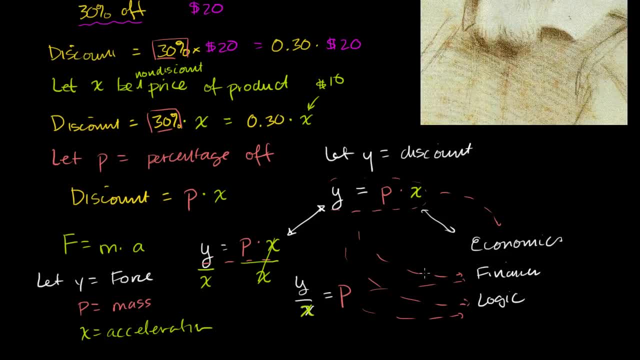 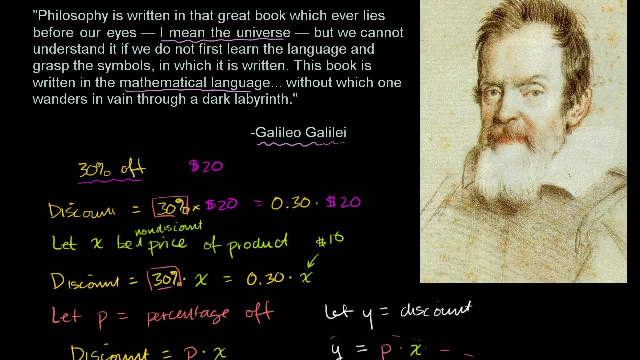 And we don't even know, frankly, most of them. We're going to discover new ones for them in 1,000 years, And so hopefully this gives you a sense for why Galileo said what he said about really mathematics is really the language with which we can understand. 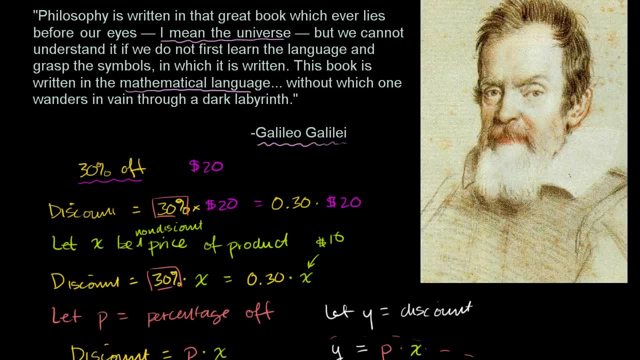 the philosophy of the universe, And that's why people tell us that if a completely alien life form were to ever contact humans, it probably. mathematics would probably be our first common ground, the place that we can start to form a basis that we can start to communicate from.